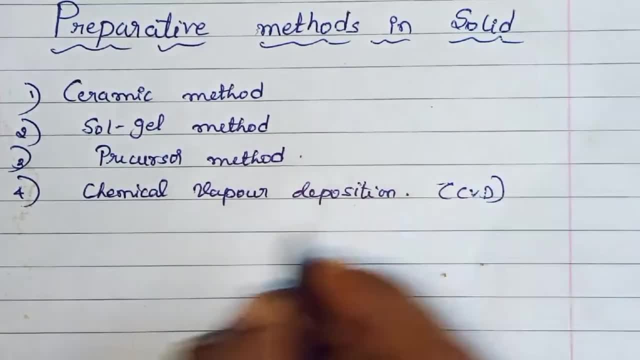 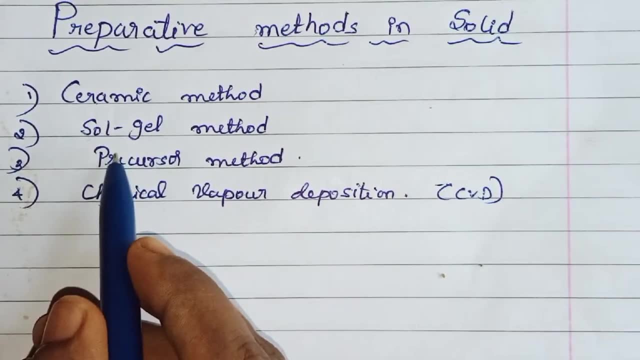 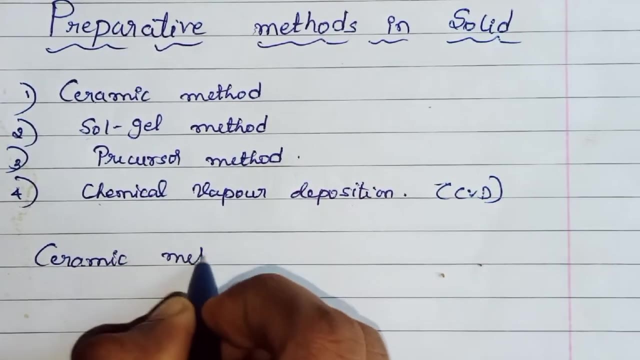 or this can be called as CVD also. Okay, and in this video we will study about the first method, that is, the ceramic method, and other three methods we will see in the upcoming videos. Okay, so we will focus on ceramic method now. Okay, now, the ceramic method means: 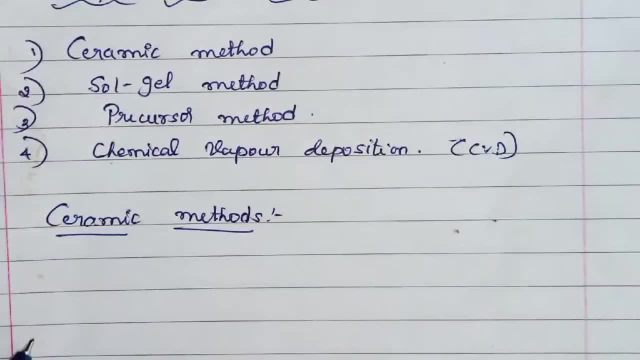 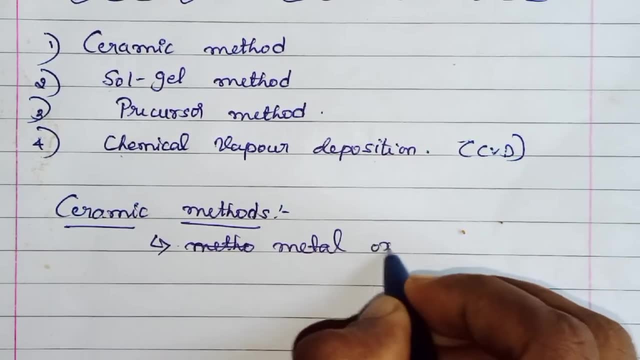 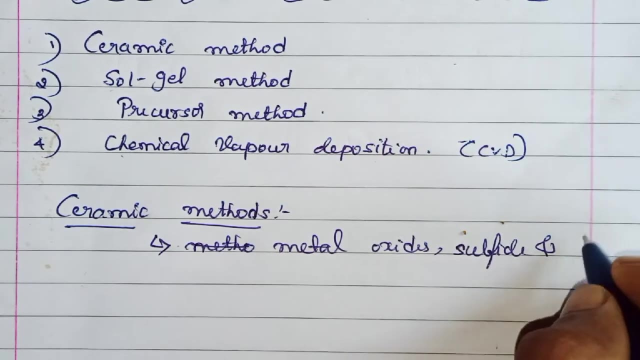 by this method. what we can prepare is: we can prepare metal oxides- Okay, we can prepare, sorry, the metal oxides, as well as we can prepare metal sulfide And the metal phosphides. Okay, by ceramic method. what we can prepare, we can prepare. 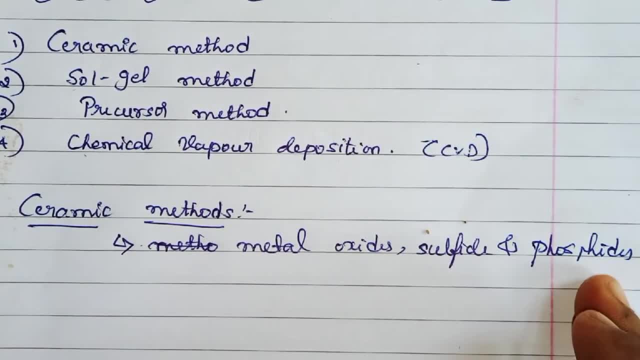 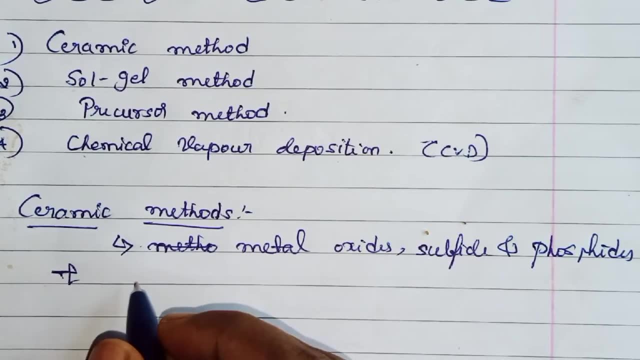 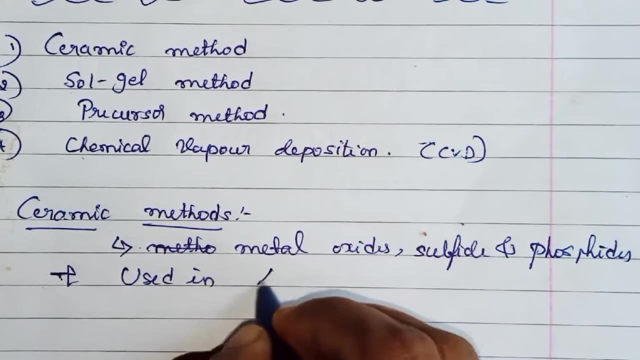 the metal oxides, metal sulfides as well as metal phosphides. Okay, in this method. okay, this method is a fine application in the industry as well as in the laboratory. Okay, it is. it is used in laboratory as well as in the laboratory. Okay, so in this method, we can. 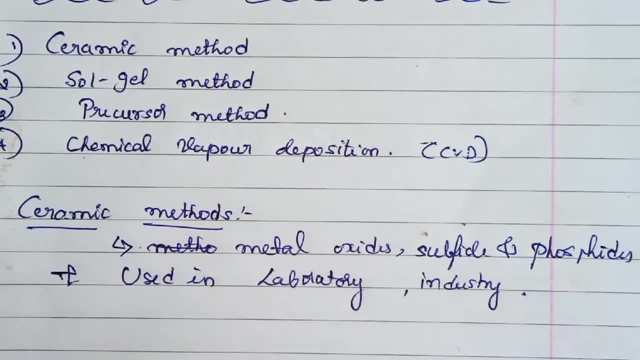 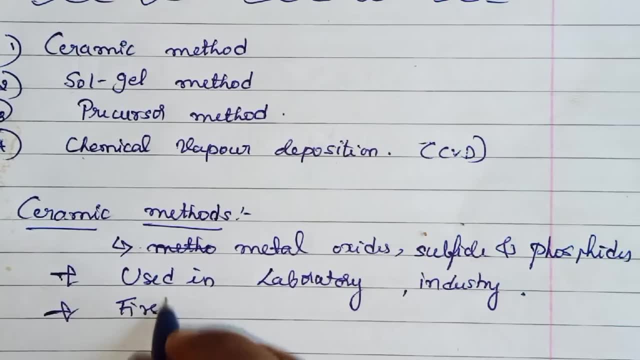 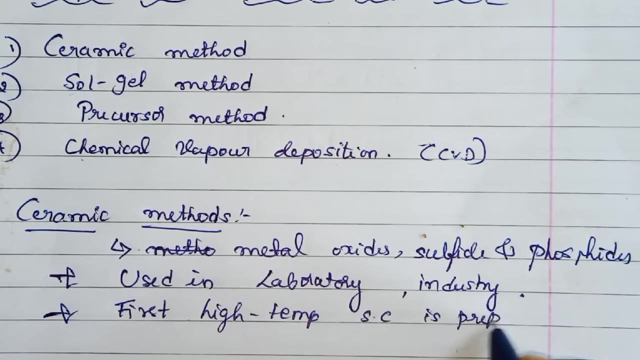 prepare the ceramic metal oxides and we can prepare the Infinity-Destined-Ceramic reported in the industry. Okay, The first high temperature superconductor was prepared by the ceramic method. Okay, the first high temperature superconductor is prepared by ceramic method. Okay. 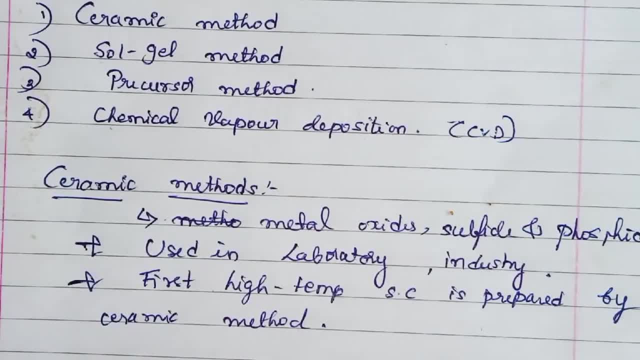 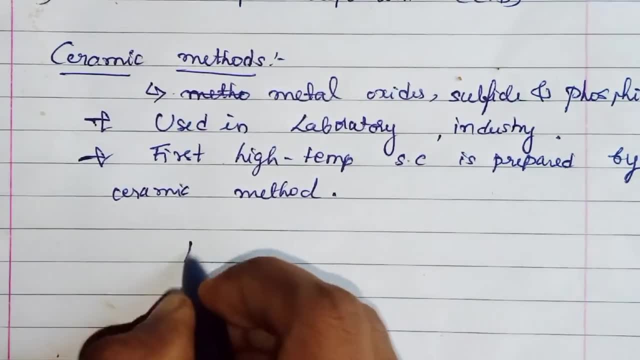 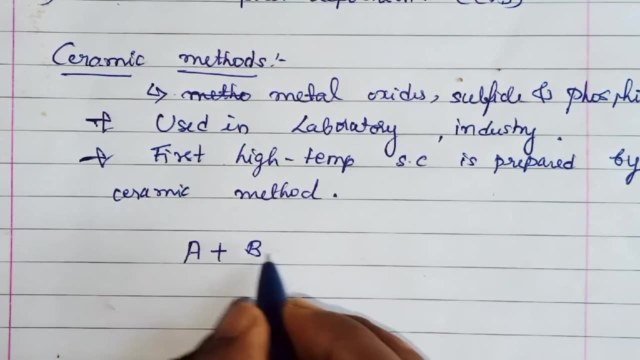 Now, the now to prepare the solid by this ceramic method is very simple. okay, the first. first, what we need to do is we have to take the starting materials that are solid. okay, just imagine a and b are the starting material. okay, both are solid. and remember, these two are non. 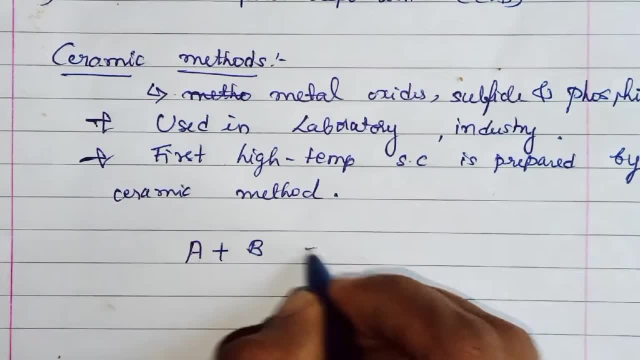 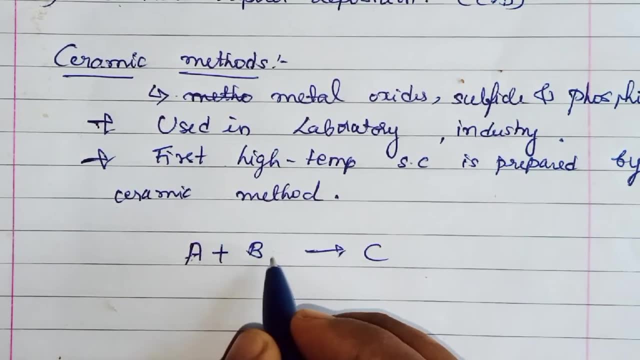 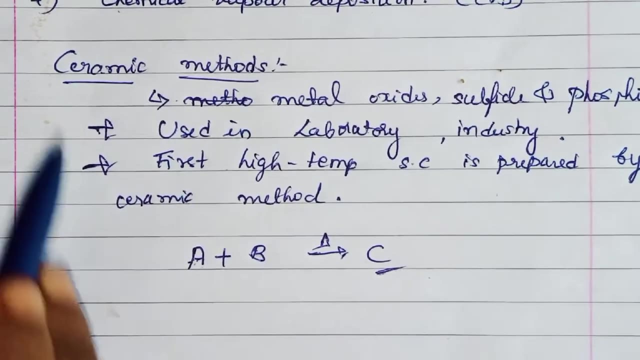 volatile solid starting material. now, if you want to get the product, say c is the product. okay, now what you need to do is just take these two, a and b, in the stoichiometric ratio and then just heat it. you will get the product. okay, such a simple method is this ceramic method. okay, we can prepare. 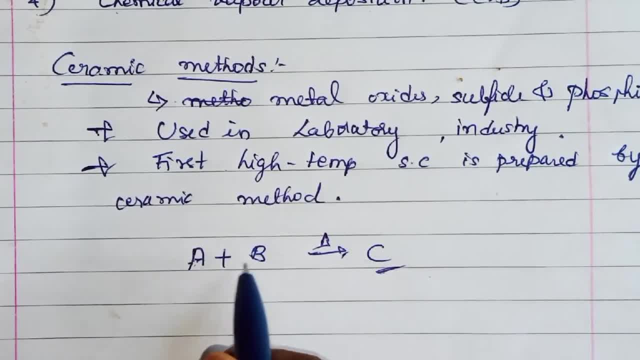 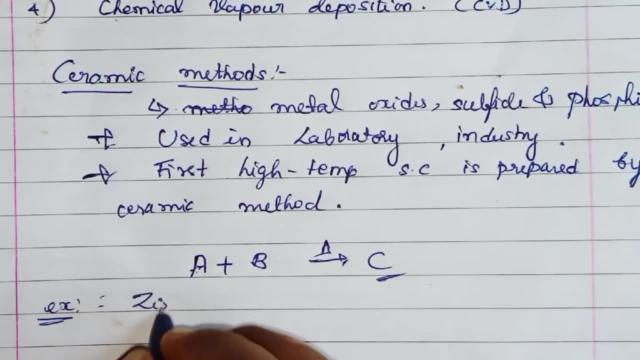 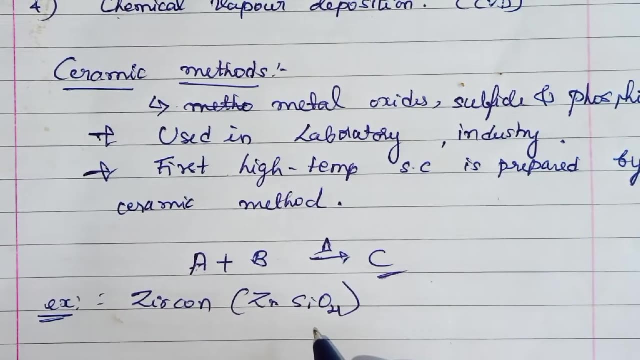 our solid material just by heating the starting material. okay, we will take the example. the example is a zircon. okay, the zircon, the formula is z r s i o 4. okay, the zircon is nothing but a gemstone. okay, that means it find application. 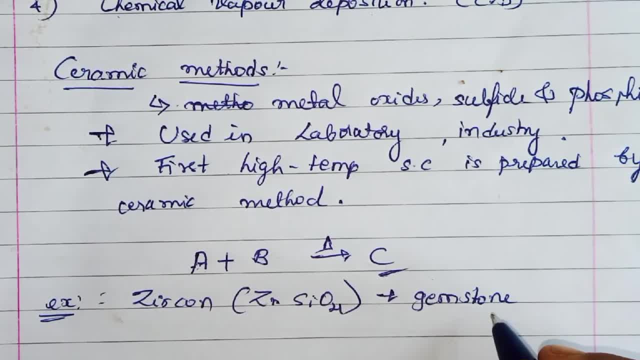 the manufacture of ornaments. okay, like, um, like jewelry, or maybe rings. okay, people believe that if they wear such uh ornaments, uh, it will bring them a wealth, or it may bring them health, health, okay, such stones are called as gemstones or zircon. okay, now to prepare this zircon. 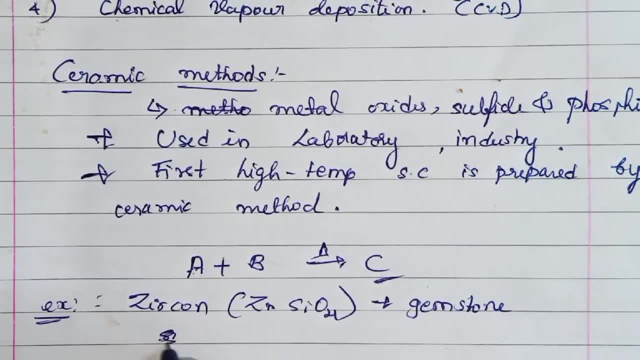 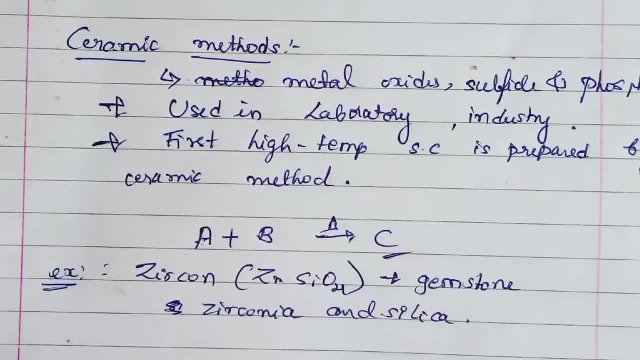 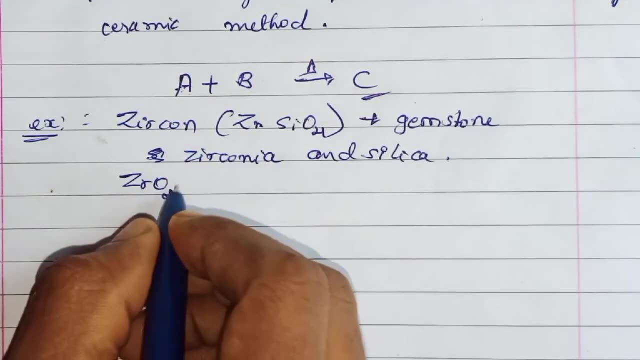 the starting materials are zirconia, the zirconia and silica- okay, these are the two starting material to get the zircon: okay. zirconia formula is zr o2- okay, it is in the solid state. and silica is si o2- okay, both are in the solid state and 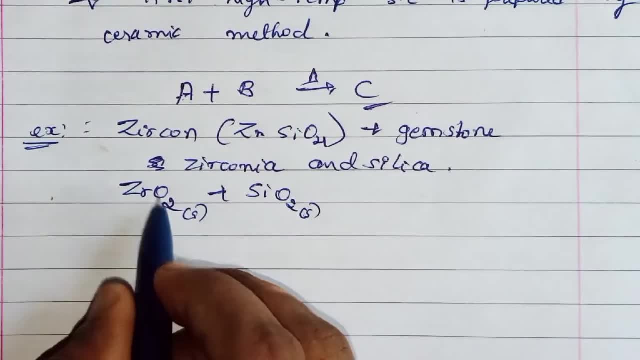 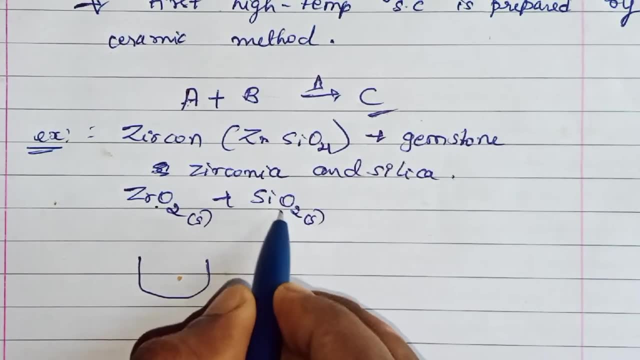 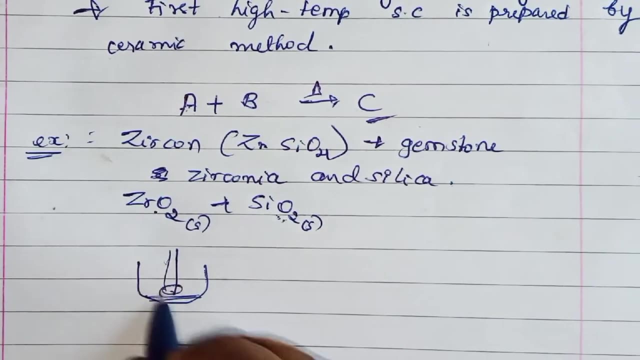 both are non-volatile. okay, first, what you need to do is you have to take zirconia in some crucible and then you have to take this one that is silica. then what you do is just grind them by using pestle and mortar. okay, just grind them using pestle and mortar so that you 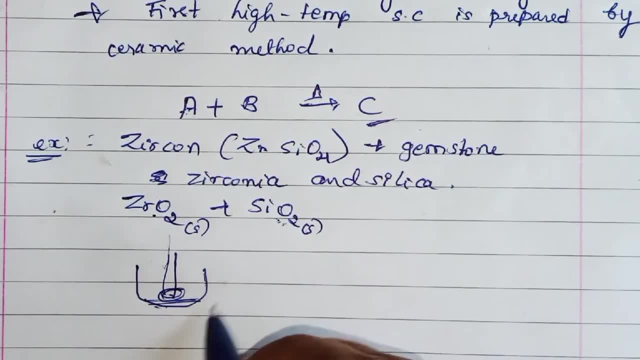 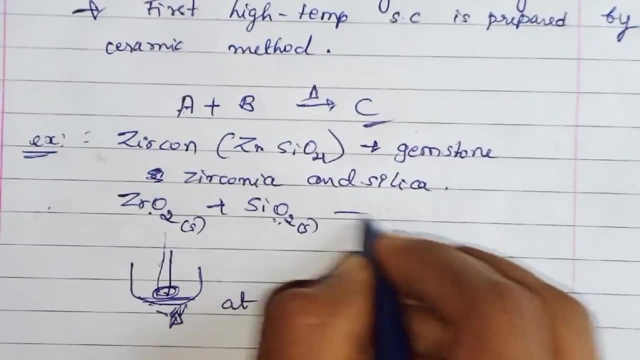 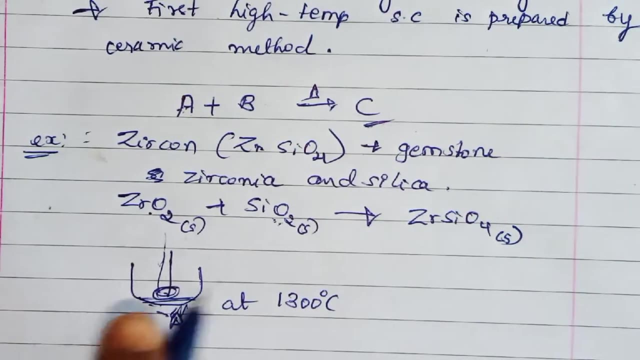 will get the fine powder. then what you do is you just heat it. okay, just heat it at the temperature of 1300 degrees celsius so that you will get your product, that is, zircon, zr, si, o4. okay, this is also in the solid state, okay, first, what you need to take. you have to take zirconia, okay, and silica in. 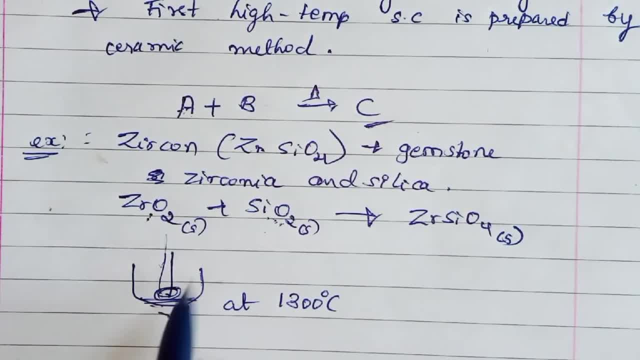 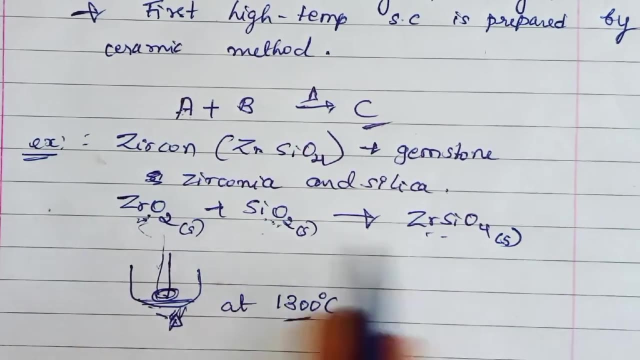 the stoichiometric ratio in some crucible, then you need to grind them so that you will get the fine powder of these two. then heat it at 1300 degree celsius so that you will get your product zircon. okay, this is zircon, this is zirconia. okay, don't get confused with these two. well, this is. 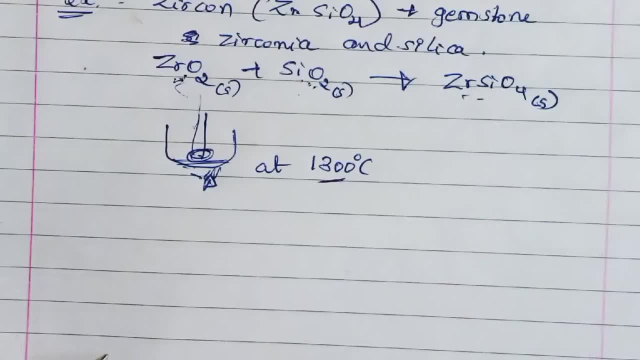 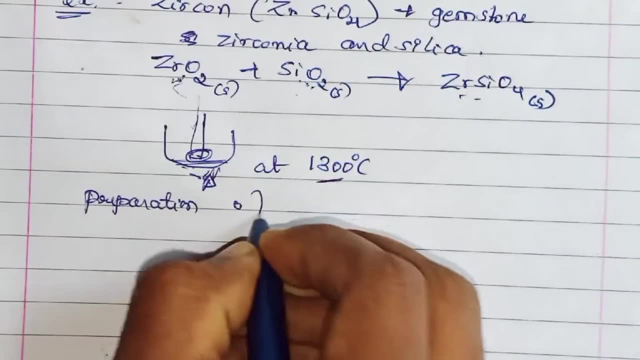 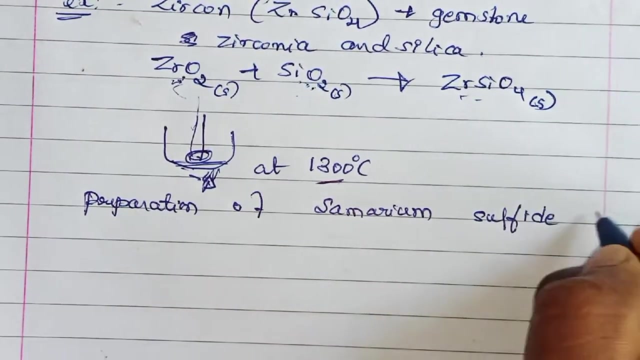 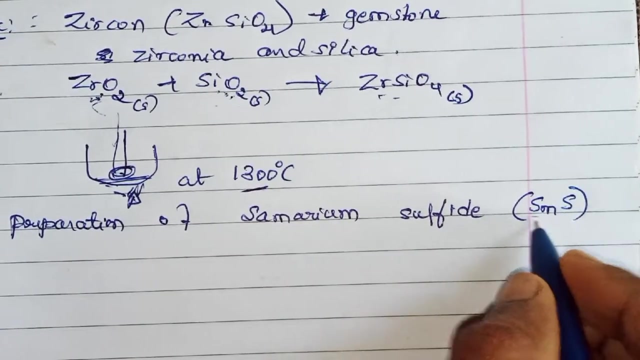 the first example. the second example that i will give is the preparation of preparation of making the periostecia. okay, so this is the first experiment that we will do is this is the component unit, now here in this 필 py студio, to first test. test this is say ion, right? so this? 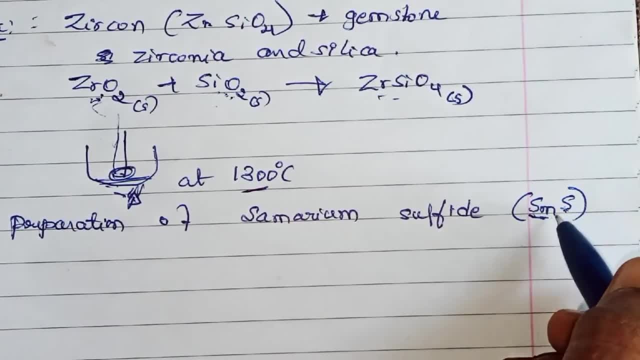 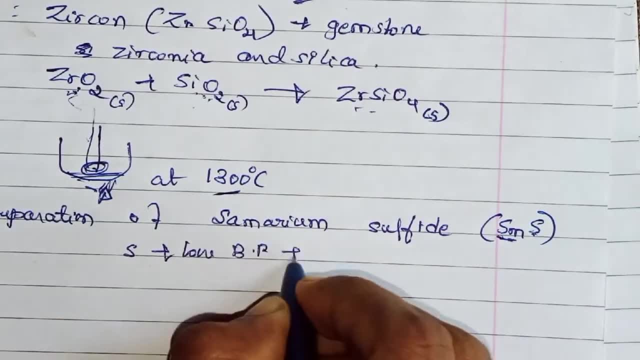 is ion. so this is ion and this desert, and also this is ion, and this is some of these- are high oxygen content and this is thegel here: 5000 k ohm. so this is the men Samanthampers right here. this is 1.2.. 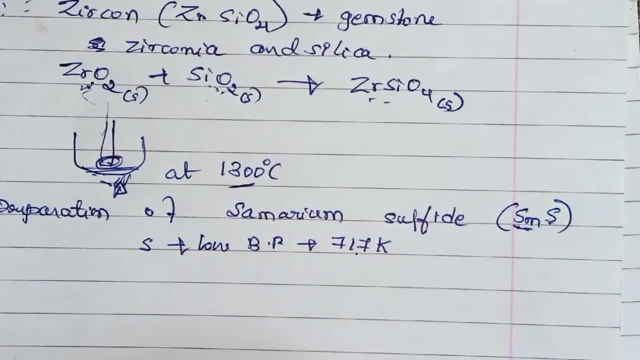 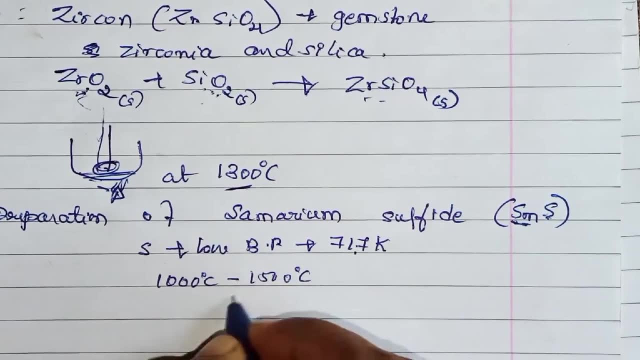 periostecia Warning sulfur. but we know that all solid state reactions happens at this particular temperature: 1000 degree Celsius to 1500 degree Celsius or more than this. okay, it always takes place at temperature above 1000 degree Celsius. okay, solid state reaction always happens at very higher temperature. 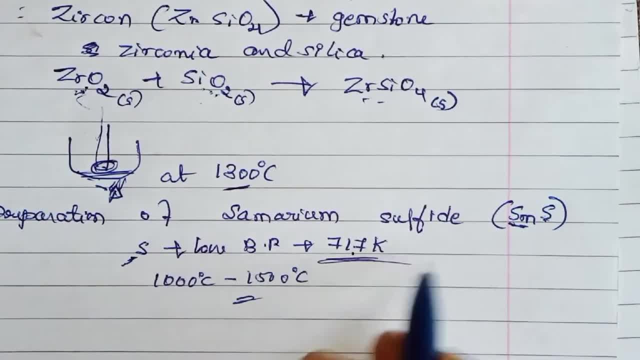 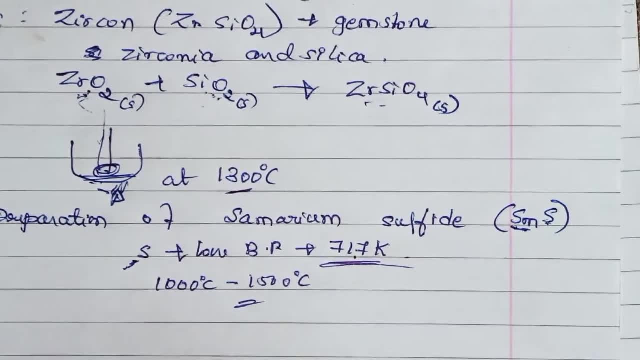 but if you see here sulfur, it has very, very lower boiling point, that is 777. so there might be possibility that that this sulfur may sulfur may boil off whenever you heat it. so to preserve this sulfur you have to use some evacuated chamber. okay, evacuated chamber is used. why? 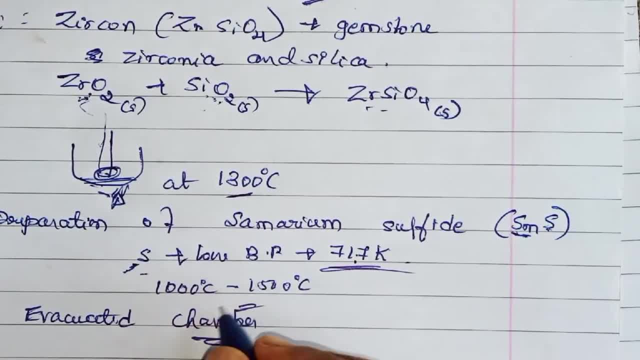 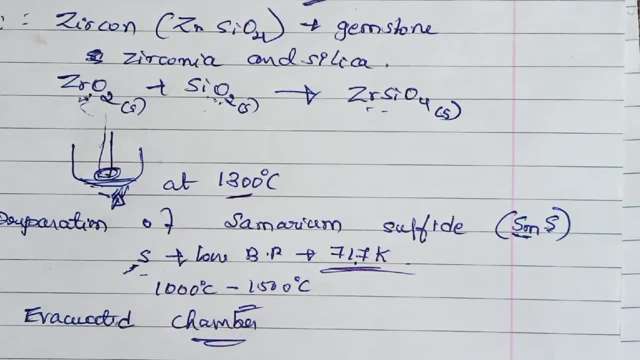 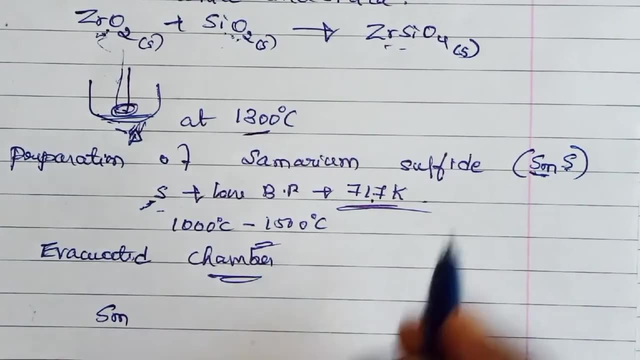 because sulfur is having very lower boiling point. so that if we heat the samarium and sulfide, what happen? there is a chance that sulfur may boil off. okay, that is the reason why we have to use evacuated chamber First. why What you need to do is you have to take samarium. okay, starting material is samarium and sulfur. 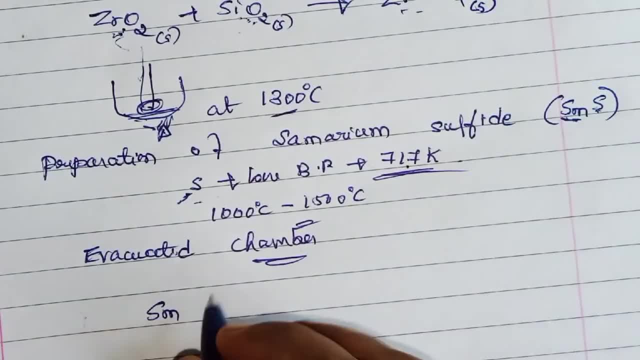 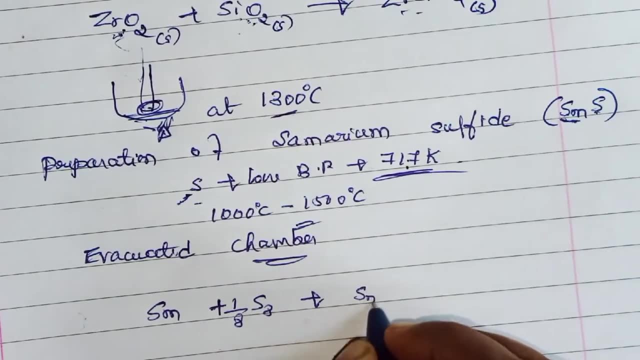 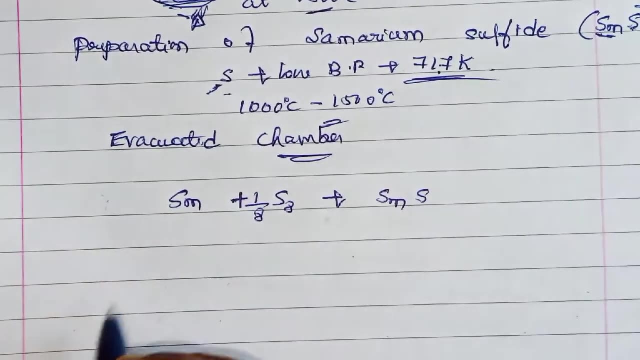 as already told, first you have to take some samarium and sulfur. okay, samarium and sulfur, they are taken in the stoichiometric ratio so that you will get samarium sulfur. the first method or first step in this is you have to take samarium and sulfur. okay, you have to. 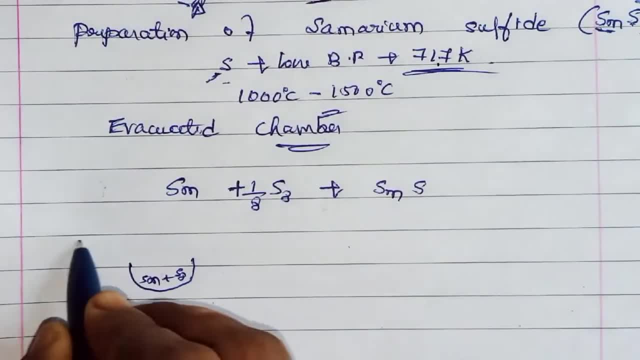 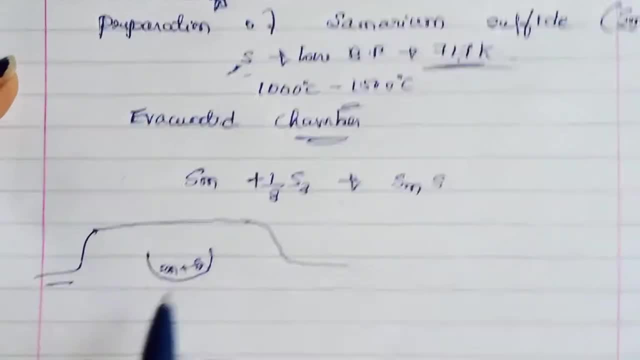 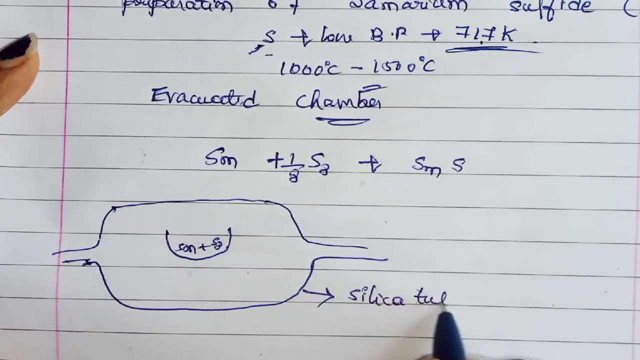 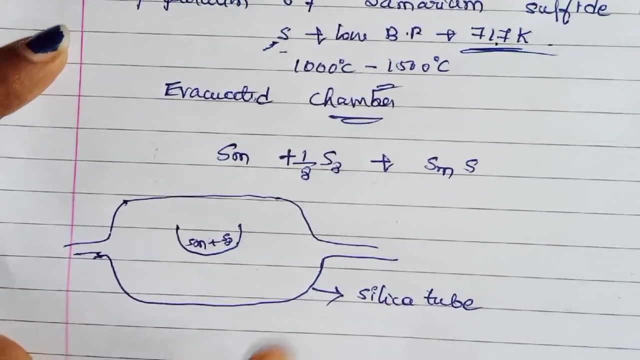 take it in a stoichiometric ratio And then you have to heat it in the silica tube. okay, you have to take that in the silica tube. Okay, this is the silica tube. okay. Okay, this is a crucible. usually alumina is used to be crucible. okay, and here you have. 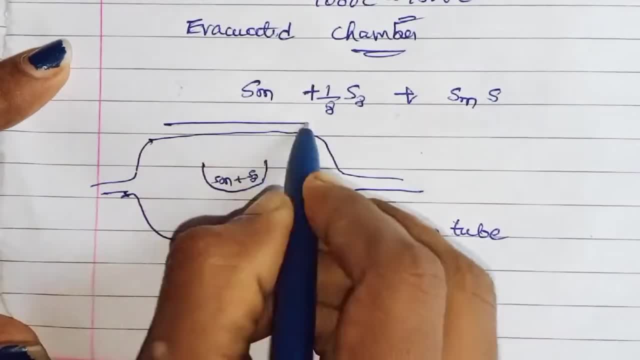 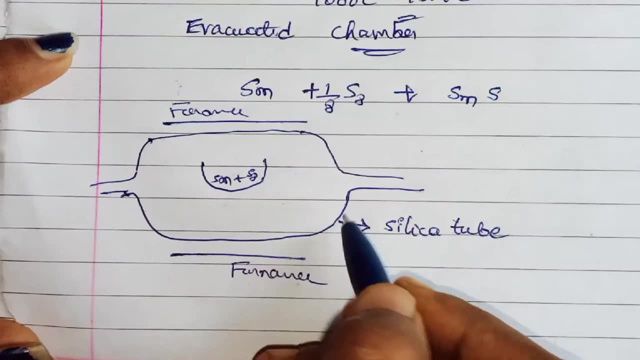 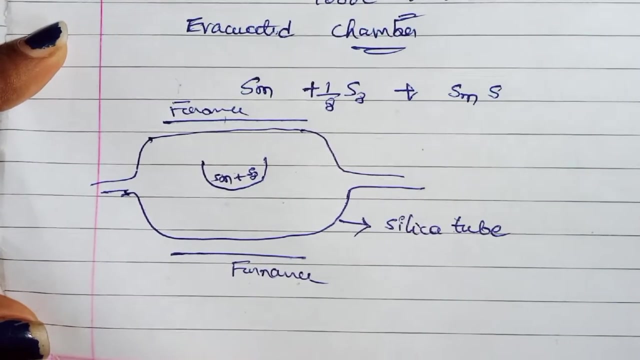 the furnace. okay, furnace. So this is the furnace, This is the furnace, This is the furnace. This is also a furnace. okay, you are just keeping the silica tube in between the furnace. Then what you are doing is you are heating that mixture of samarium and sulfur at the 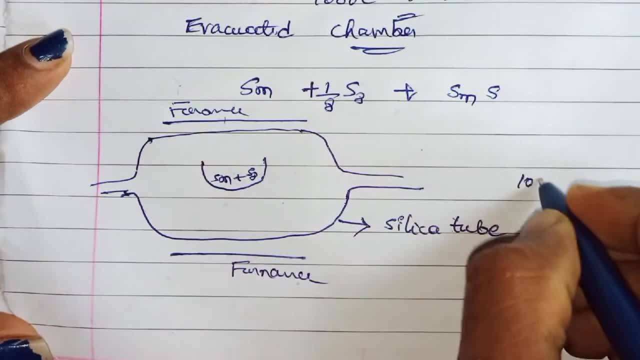 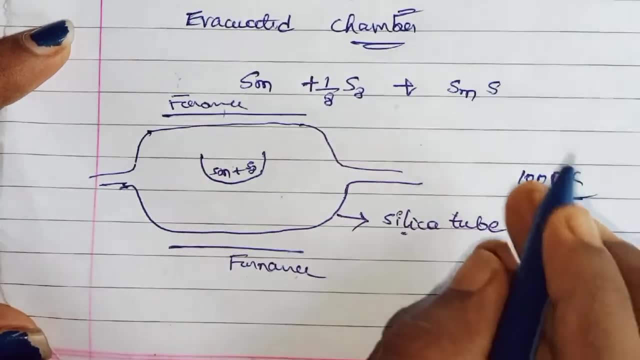 temperature of 1000 kelvin. okay, at what temperature you have to heat 1000 kelvin? In what? in the silica tube you have to heat that at this particular temperature. Then you, after several hours of heating at this particular temperature, then you need. 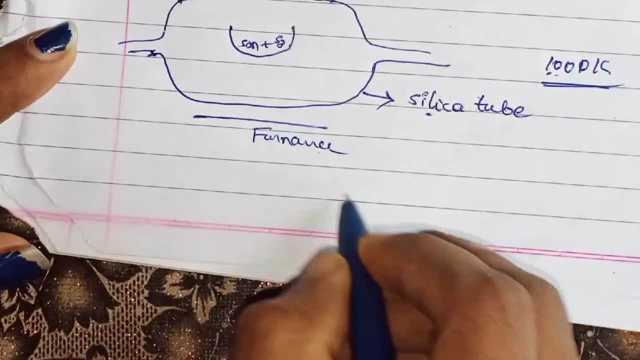 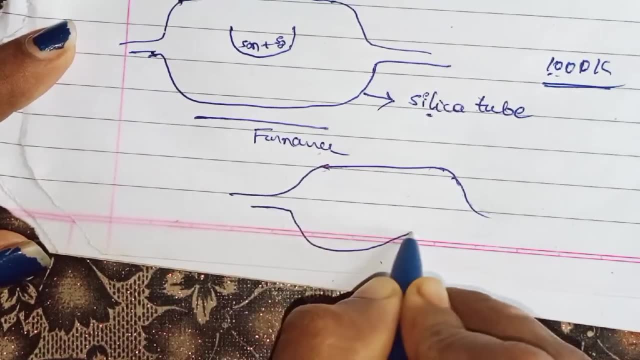 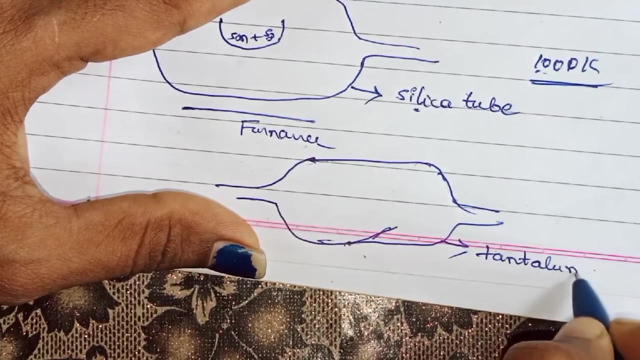 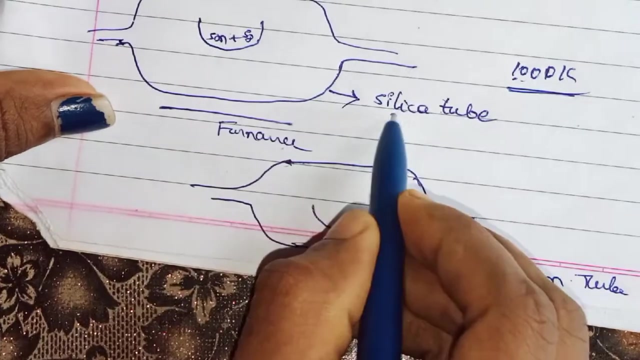 to remove this crucible, And then you keep the same crucible in the tantalum tube. okay, okay, this is the tantalum tube. okay, I am just keeping the same crucible. okay, here I heated the crucible in the silica tube at 1000 kelvin and then what I did? I just removed the crucible by this silica tube. 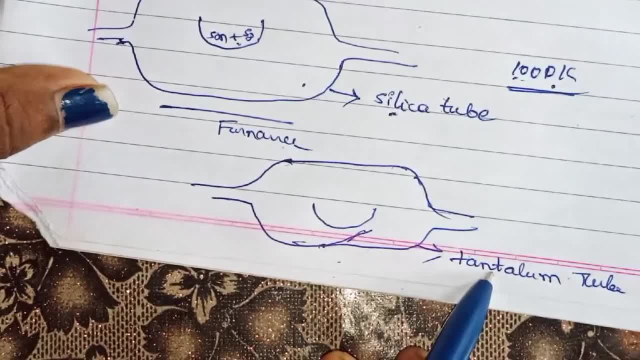 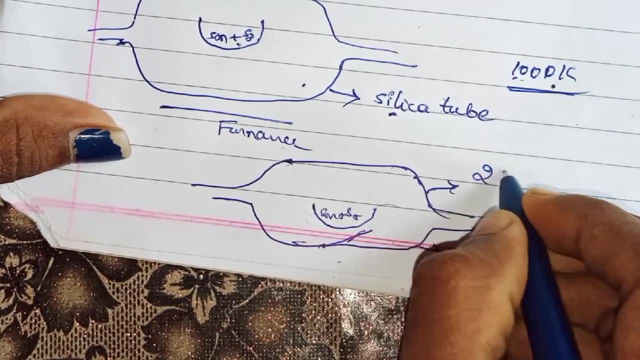 Then I placed it in the tantalum tube. Okay, Okay, In the tantalum tube. okay, I have the samarium and sulfur in this crucible also, and this time I am heating at at 2300 kelvin. okay, in the tantalum tube, I am heating this crucible. 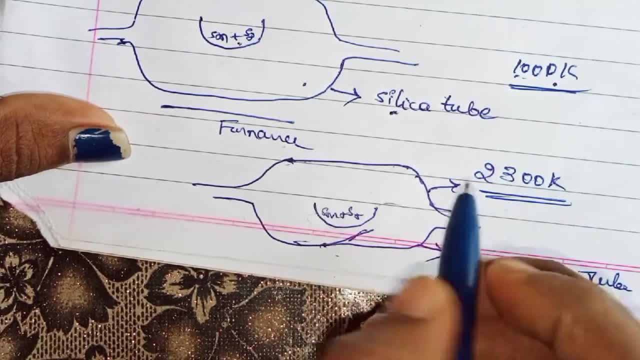 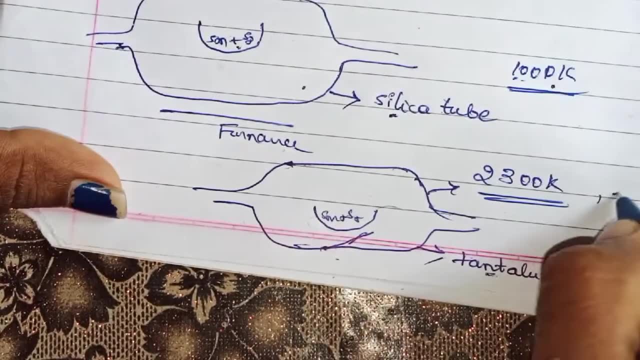 at 2300 kelvin. and this time we are not using the furnace. okay, here we use the furnace, right, but here we are not using the furnace. instead, electricity is used. okay, instead, what is used? the electricity is used to use it for the furnace. Okay. 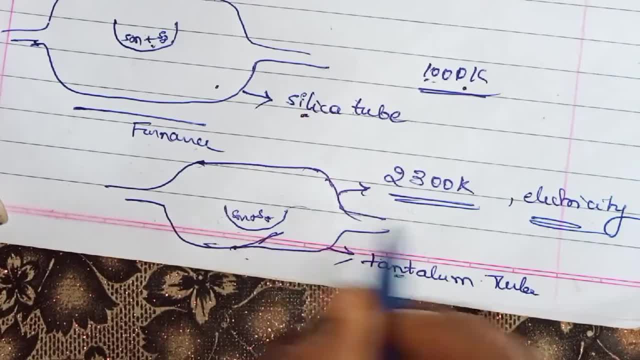 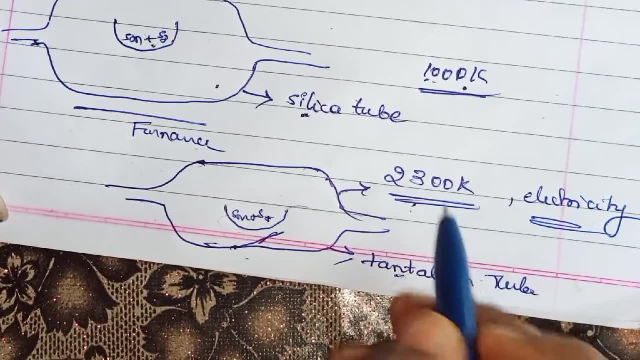 Okay, We have to use it for the heating of this crucible at this particular temperature, Okay, And after heating for about like two hours or three hours like that, then you remove this. you will get your product, that is samarium sulfur. okay, samarium sulfur- okay. so this is. 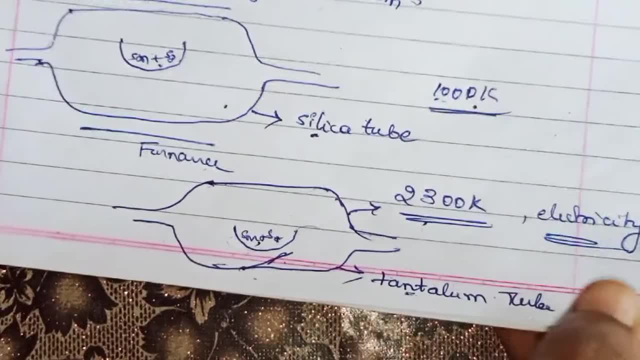 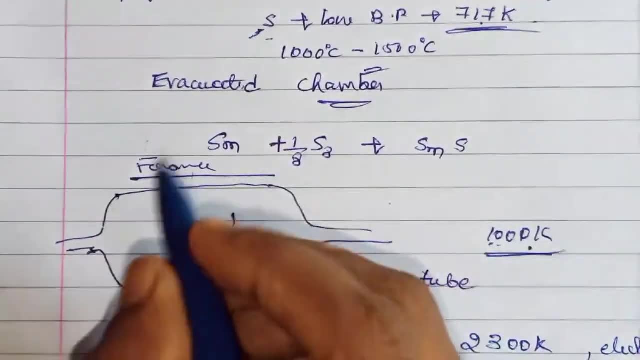 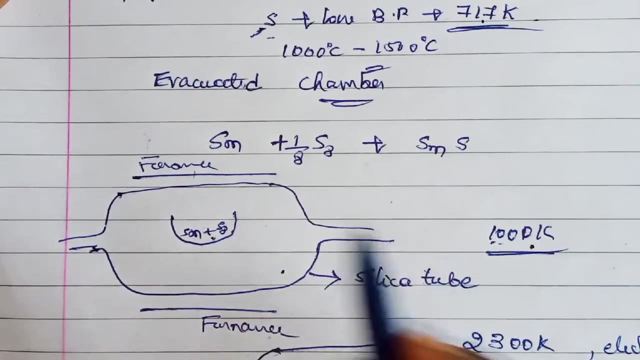 how you are. you know preparing samarium sulfur by using the ceramic method. okay, first step, what? what is the first step? first step is that you have to take a samarium and sulfur in the stoichiometry ratio, then you have to keep it in the silica tube and, by means of furnace, you 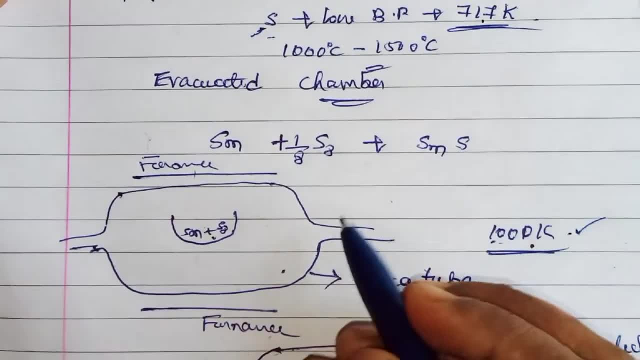 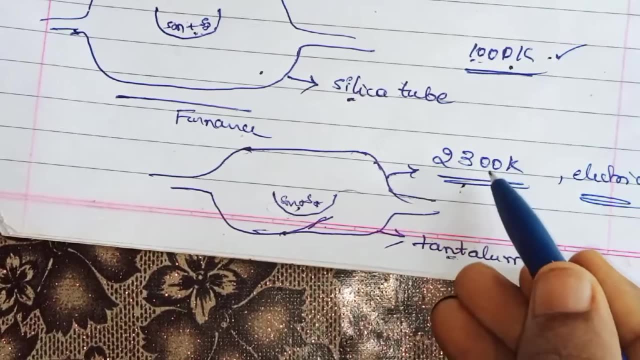 are heating it at 1000 Kelvin and after several hours of heating, remove this crucible and then keep it in the tantalum tube, and this time you heat it at the 2300 Kelvin by means of electricity. okay, and the product that you get here? 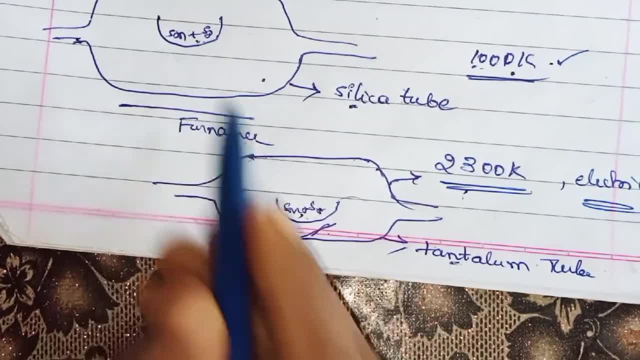 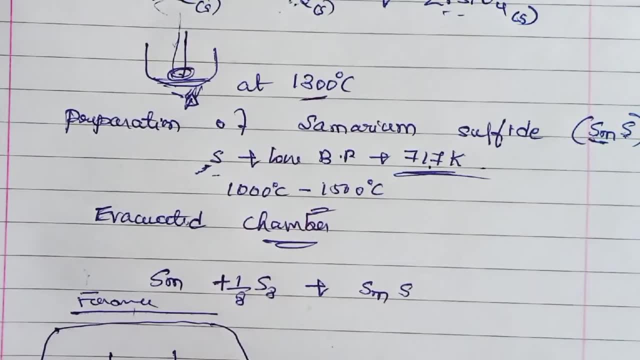 is the samarium sulfur. okay, here you do not get samarium sulfur, but here you will get. okay. so this is the method- ceramic method- used to get the samarium sulfur. and also we can get the zircon or gemstone by means of ceramic method. okay,